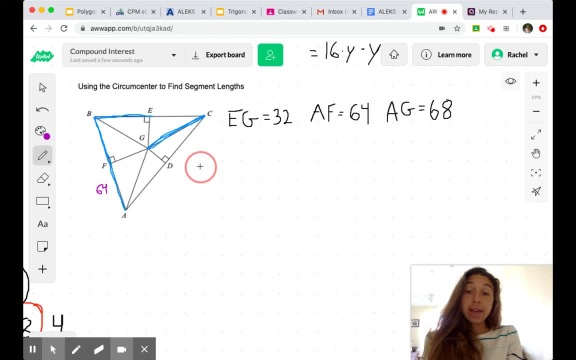 So 64 is half the length of AB, Meaning AB is 64 times 2, or 128.. Okay, We're going to come back to B. That's the one that's kind of got the most going on. We are also told that AG is 68 degrees. Now remember, every vertex is an equal distance. 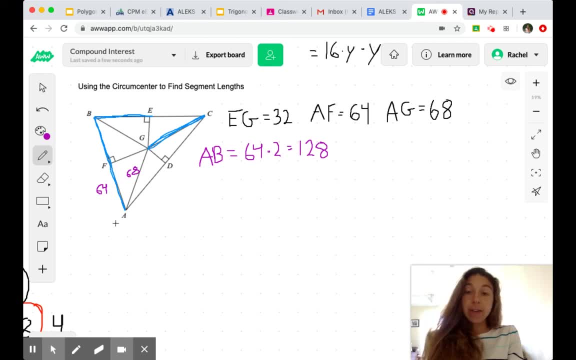 from the circumcenter. So if AG is 68, I think I said degrees, but I didn't really mean degrees- whatever unit we're using here, If AG is 68 units, CG also has to be 68 units, because C is another vertex. 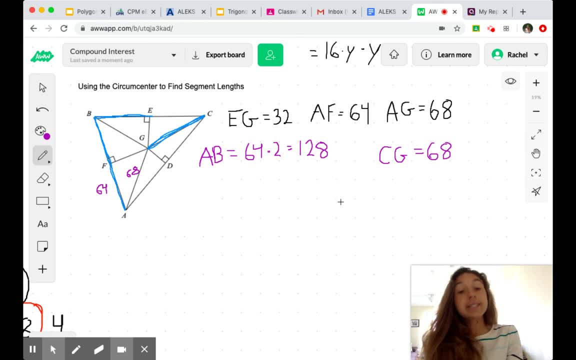 All right, And it wouldn't be fun if we didn't do at least a little bit of some computation. What else do we know? Well, we know that B is 68. So we know we need to find BE. We know that EG is 32.. 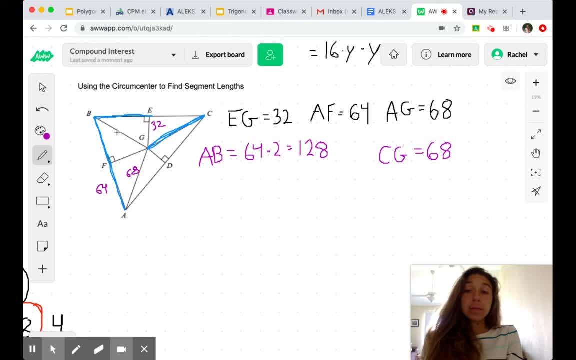 And we know BG because B is our third vertex. So we know that length is 68. And what can we use once we know two lengths of a right triangle? Hopefully you're thinking Pythagorean theorem, Because that is absolutely what we are going to use here. 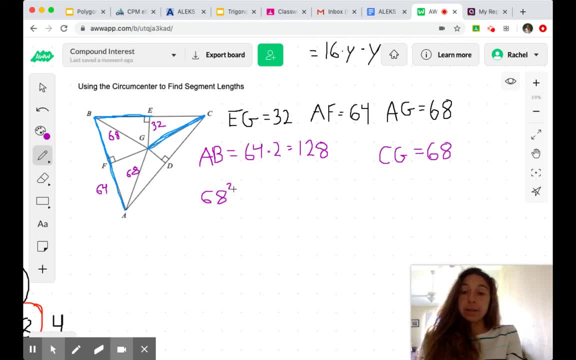 68 is our hypotenuse. So we know 68 squared equals BE squared Plus 32 squared. So we know we need to find BE squared And we know BG is 32.. there we're computing, And if you want to skip this step and go, you know kind of right.